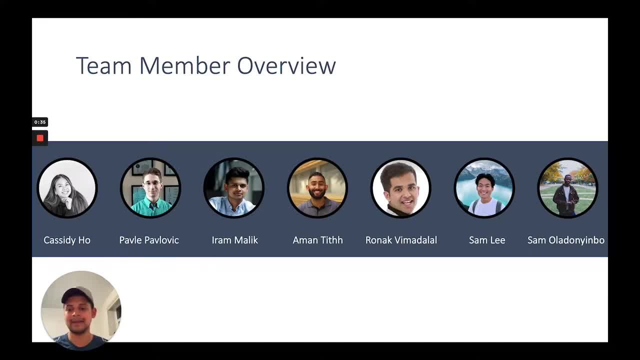 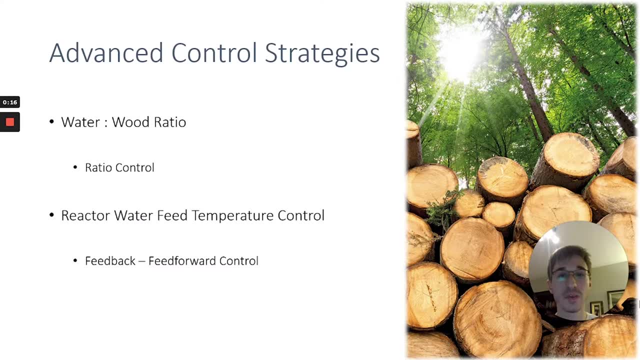 And here are all of my awesome teammates. Let's get this started. So we'll be implementing a number of advanced control strategies from GB 474.. Namely, in order to control the water to wood ratio at a set point of 19 to 1, we implement ratio control- And in order to control reactor 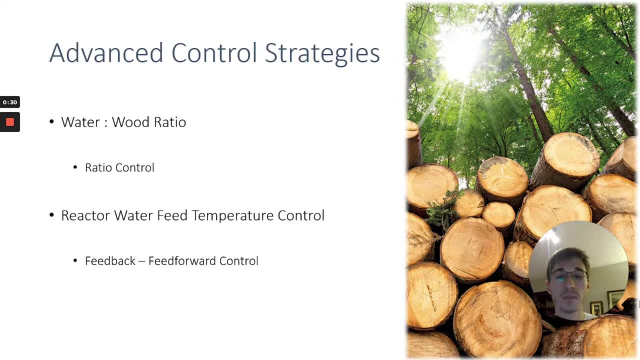 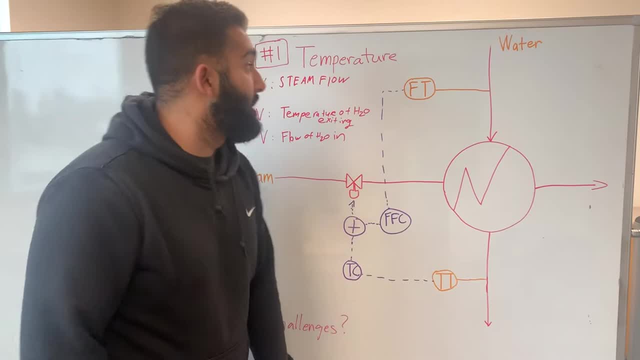 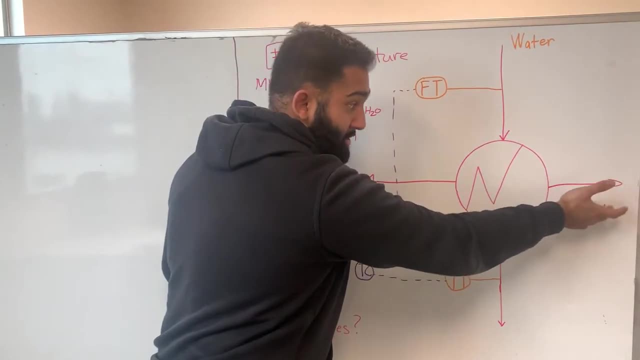 inlet temperature of the feed water. we implement feed forward feedback control. All right now onto our temperature control system. We do a quick P&ID of the heat exchanger. We have water entering here and steam entering here and leaving through a steam trap. that's not. 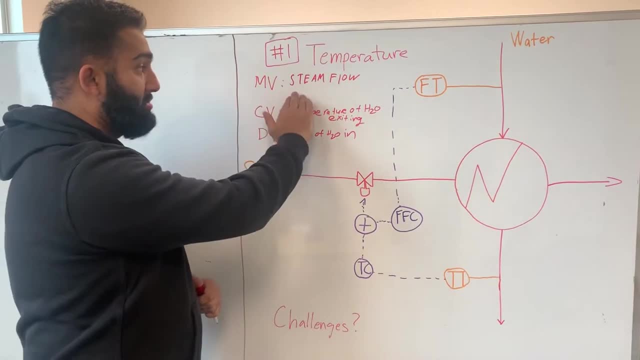 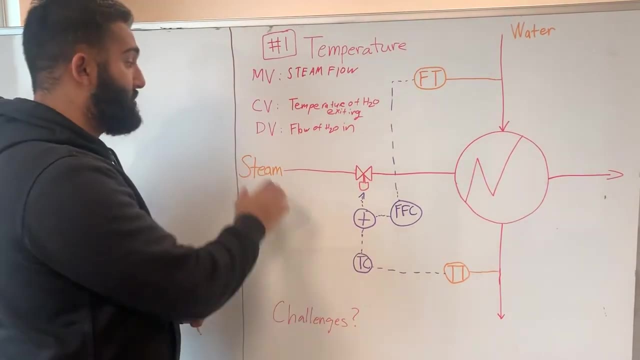 shown as condensate. So, first off, we have a manipulative variable, which is steam flow, We have our control variable, which is the temperature of the water exiting the heat exchanger, And we have a disturbance variable, which is the temperature of the water exiting the 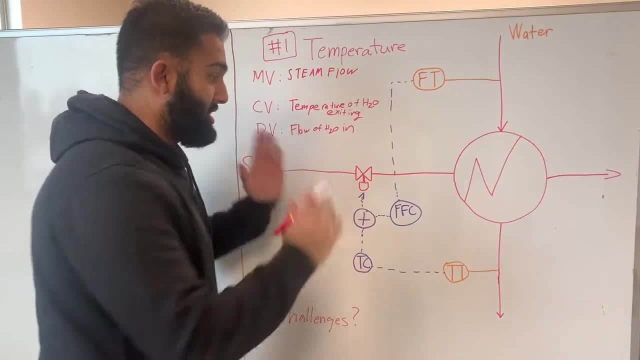 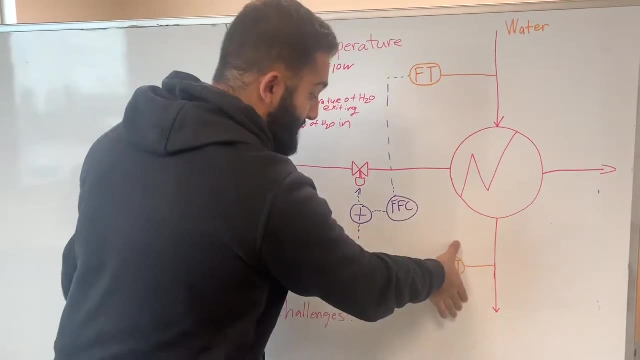 flow of the water entering, as this varies in a process. Now, quickly, the feedback. this is the feedback and feed forward system. The feedback is implemented here. the feed forward is implemented here. So we measure the temperature of the water exiting and we put that into a temperature. 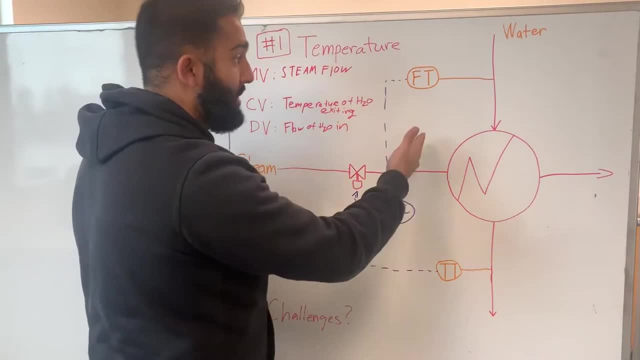 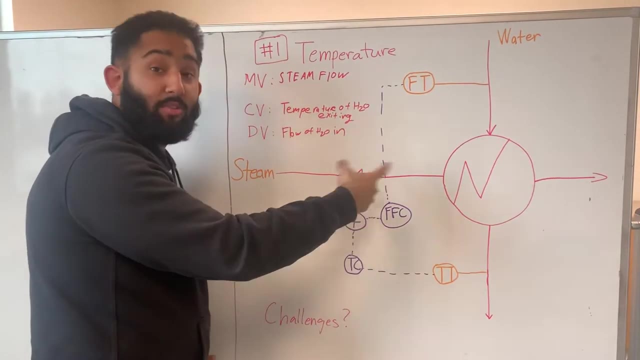 controller that adjusts the steam flow into the heat exchanger as needed. However, in addition, we also measure the flow of the water entering. put that into a feed forward controller and that also adjusts the steam flow entering to account for any disturbances in water flow. Now challenges. 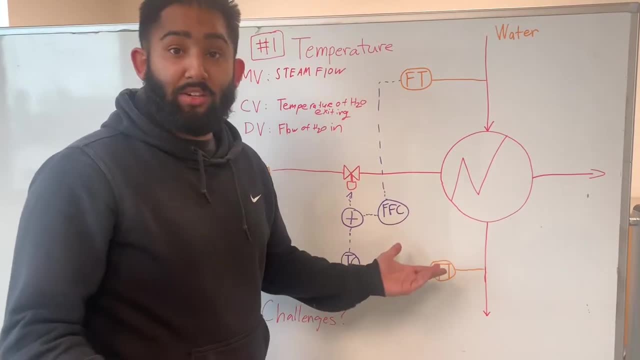 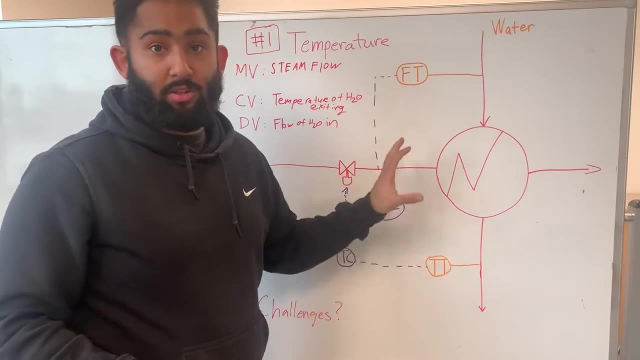 in the process are potential scaling or issues in the heat exchanger, and this feedback system helps ensure that those disturbances that are not measured are also taken care of in our control system, And of course, cascade control should be- would be thought to be implemented here. However. 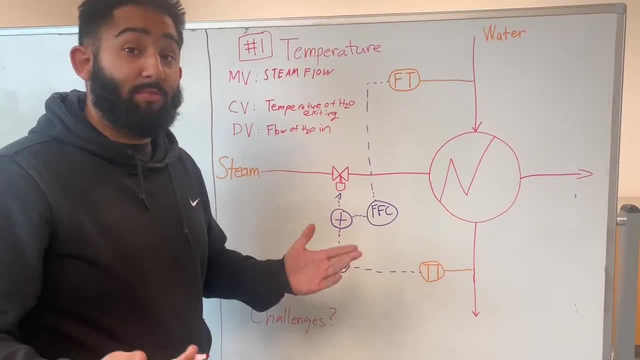 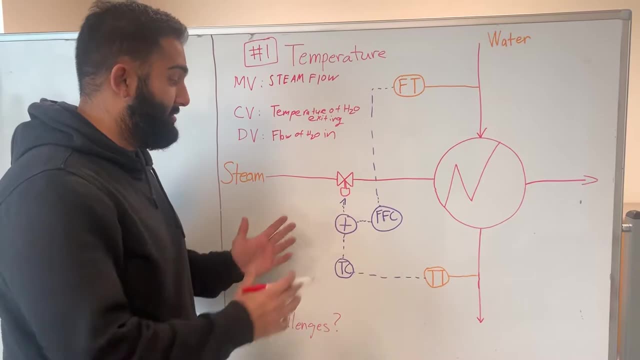 speaking of Sergio Breda, he mentioned that, since we only have one steam flow in our process, there's no need for cascade control, as the steam pressure will not vary. Therefore, to decrease the complexity of the system and just keep it cheaper in terms of 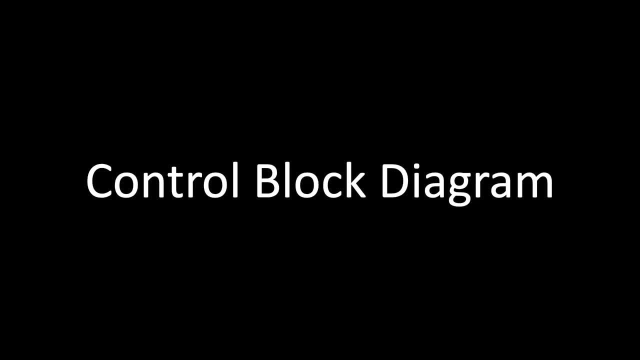 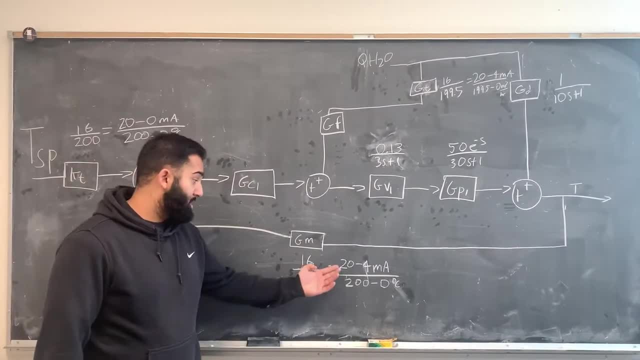 implementation. we did not implement cascade control. We have three transmitters here, here and here, For example, we determine the transmitter as we're using an electric transmitter. So there's a range between 20 and 4 milliamps and the expected range of a process is between 200 to. 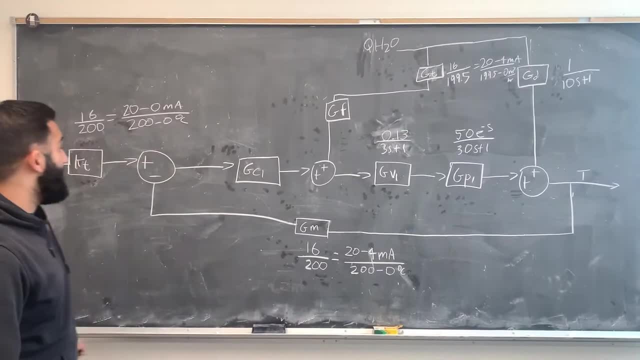 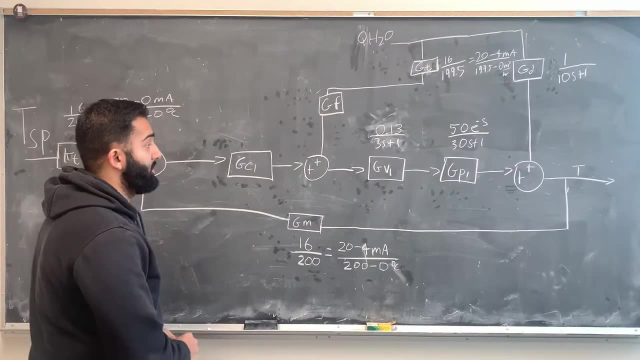 0 degrees Celsius, giving us 16 over 200.. And now we have GC1,, which will be solved for shortly, and GF, which is our feed forward controller, and that will also be solved for shortly. We have GV1,. 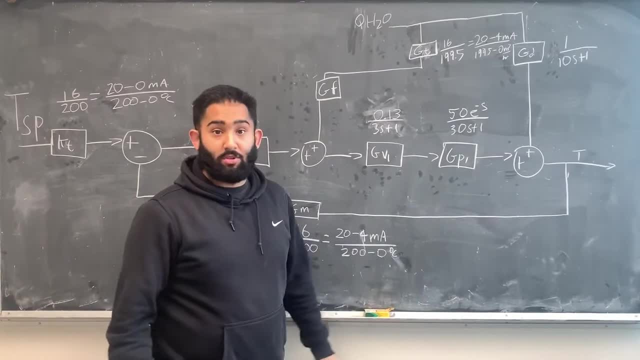 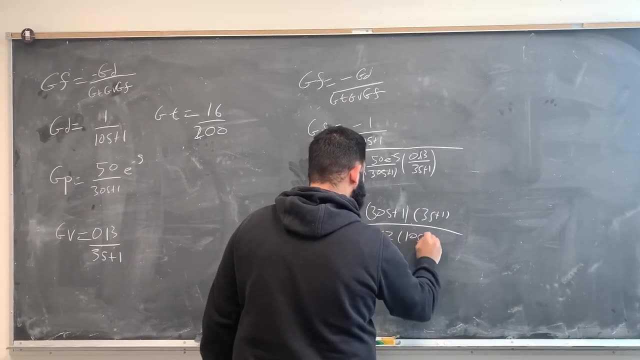 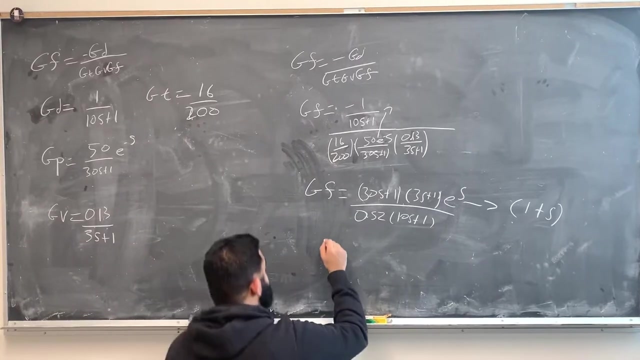 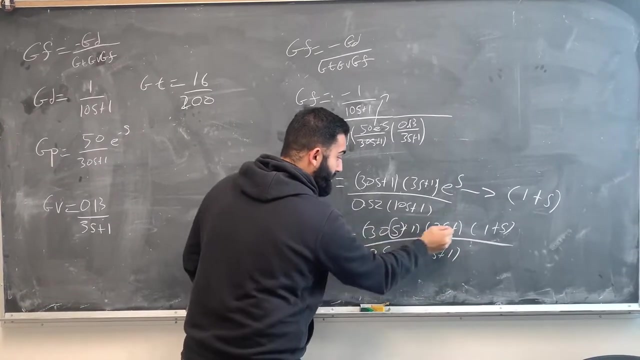 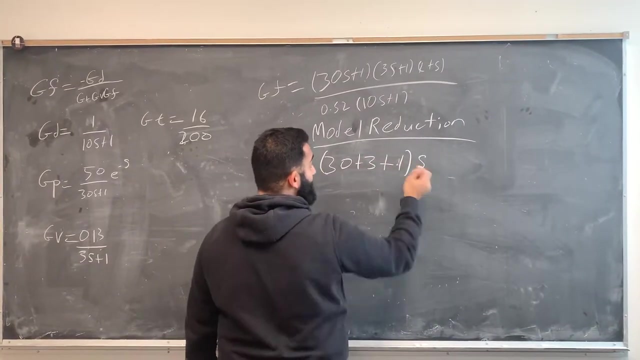 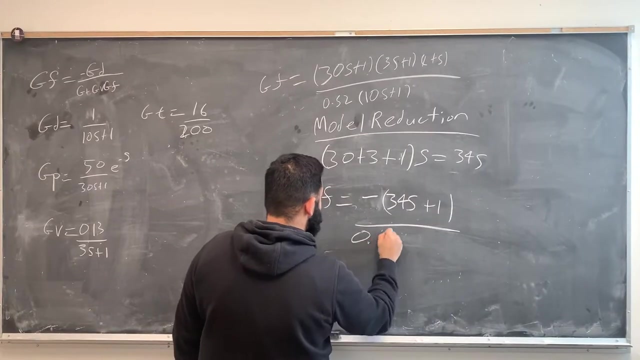 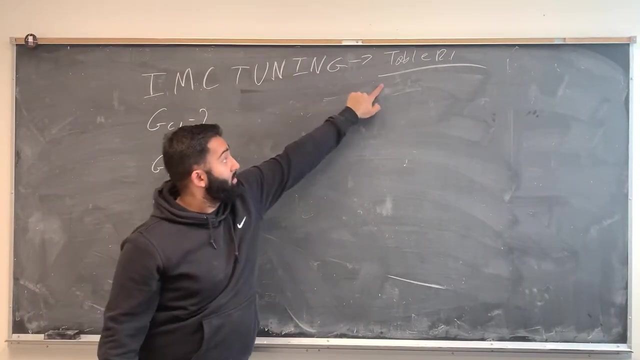 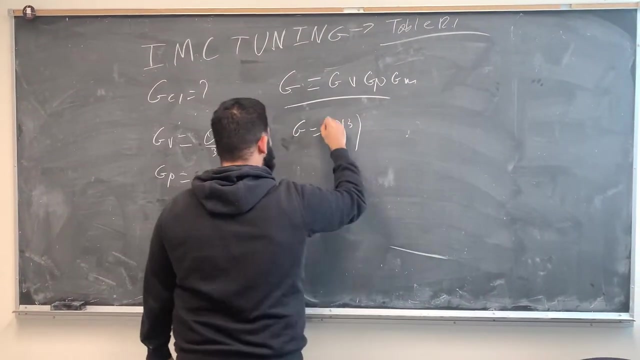 both. all three of these have got in their transfer function some literature, But with the maximum of GV1, that's just a real little bit more complicated than what we're actually doing. Speaker 1- Speaker 2. Speaker 3- Speaker 4. 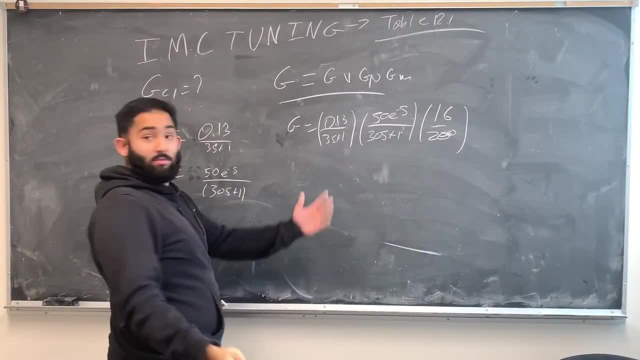 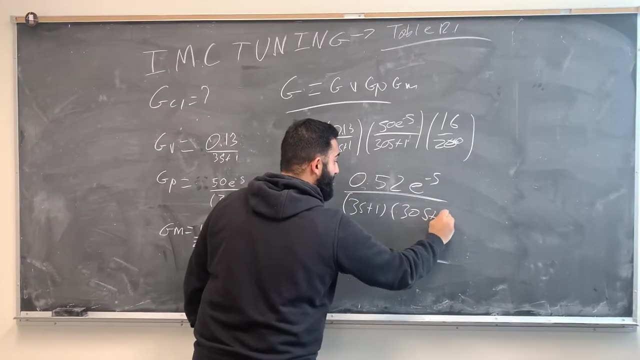 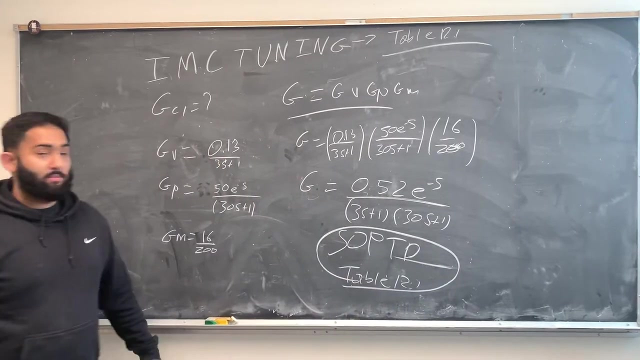 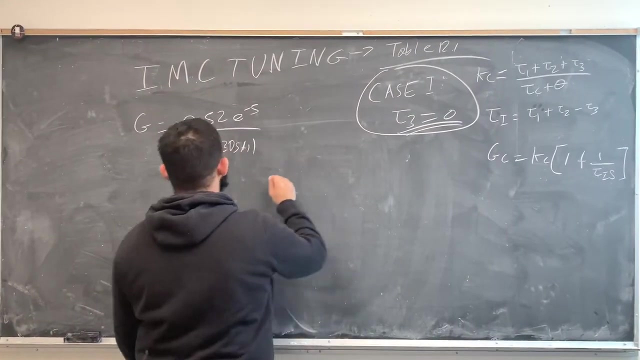 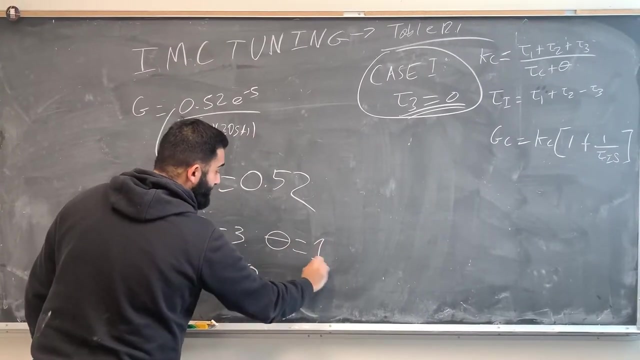 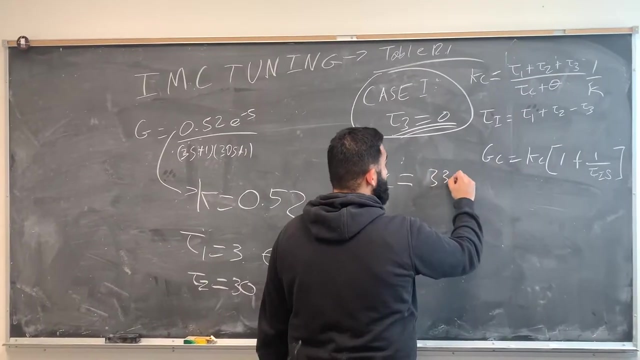 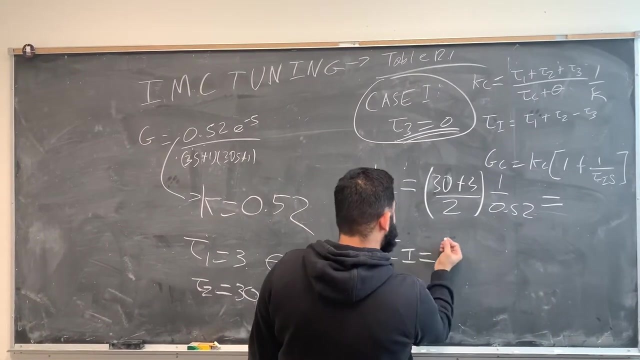 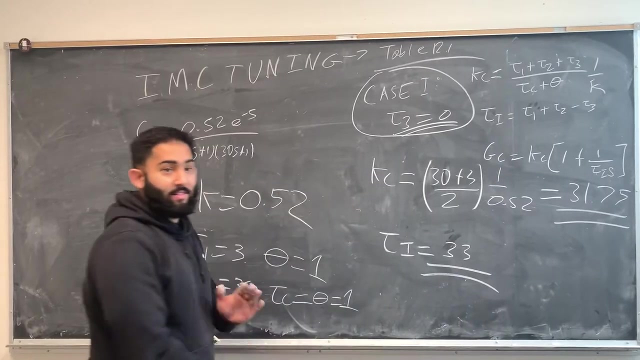 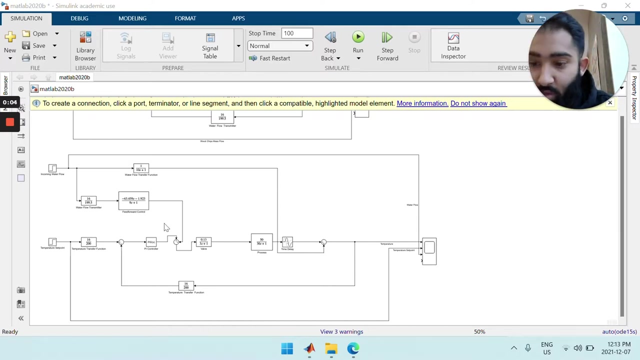 Speaker. 4 Speaker. 5 Speaker. 6 Speaker. 7 Speaker. 8 Speaker 9. Thank you, We converted that PIN ID into our Simulink file for our temperature control system. So first let's take a look at disturbance rejection. We have our set point set to 1, and with the feed forward control, implemented the response: 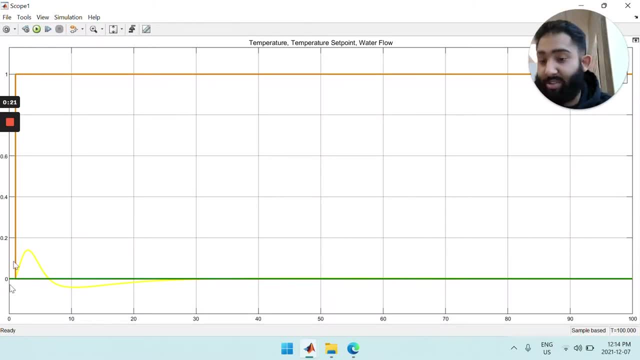 is, as seen over here, So 1 meter cubed per hour. increase in the water flow rate as a step change results in the temperature of the outlet stream to deviate slightly. However, the deviation is taken care of within 8 unit seconds and then you can see over. 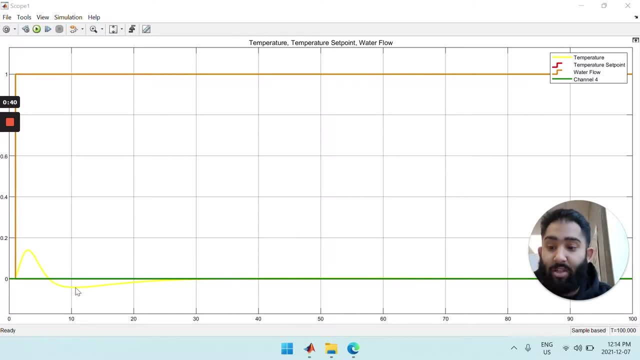 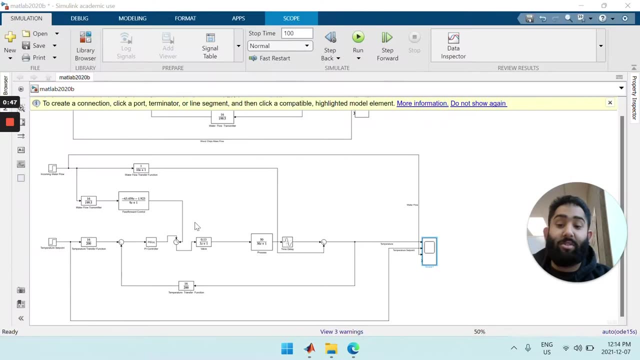 here that there is a little bit of an understeer. However, the temperature range is within steady state values. And now let's take a look at it. if the feedback control system is not implemented, So it's the same process just with feedback control. 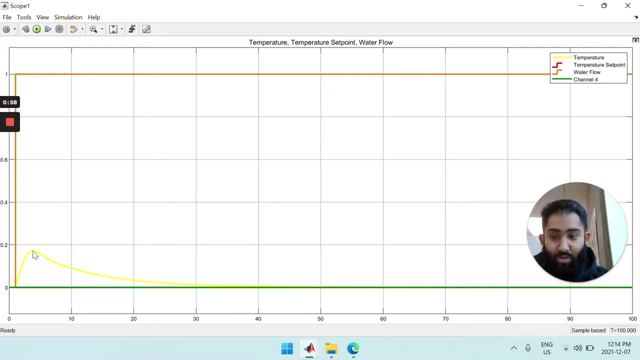 We see that the deviation is slightly larger- It's closer to 0.2, and that it is sustained for a longer period of time and takes much more time to settle down. Therefore, the feed forward feedback system as a whole helps our process. 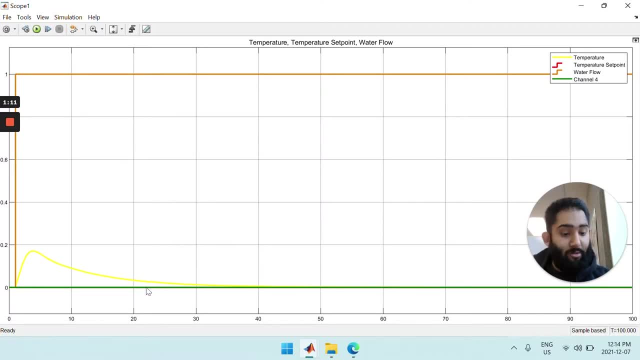 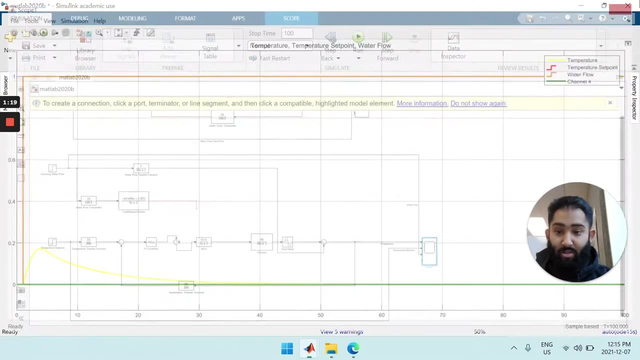 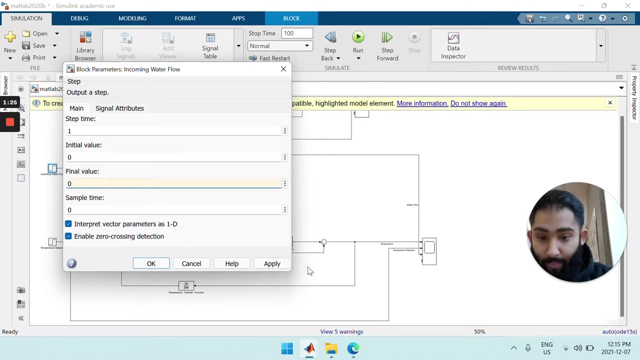 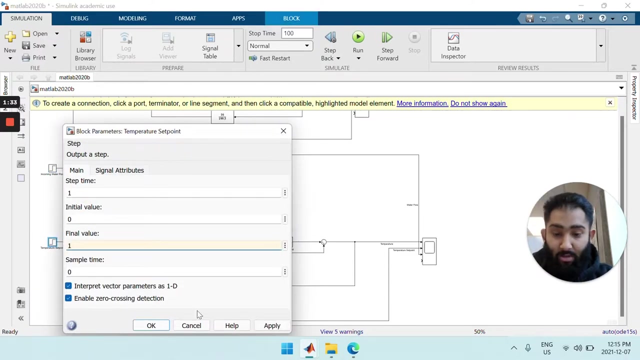 It helps us maintain the temperature of the water entering the reactor to ensure that our reactor reaction occurs at the correct temperature and the correct specifications. Now let's take a look at set point tracking of the system. So, with the say that there is an increase of 1 degree in the set point of the outlet, 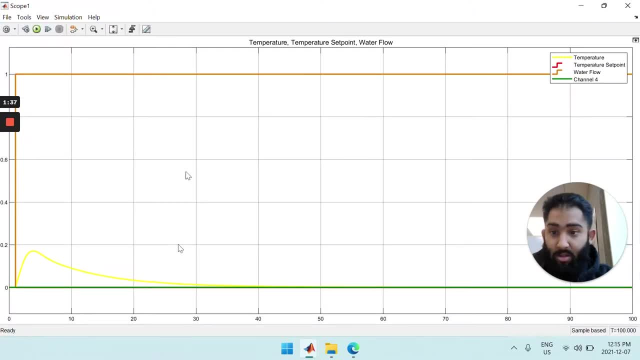 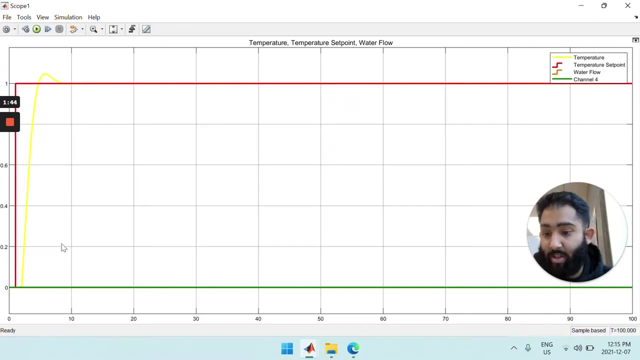 water, The Oops, The, The, The feedback controller will follow suit and the results are over here. As you can see that there is a small time delay between when the set point occurs and the action taken by the controller, as seen over here, and the temperature quickly jumps. 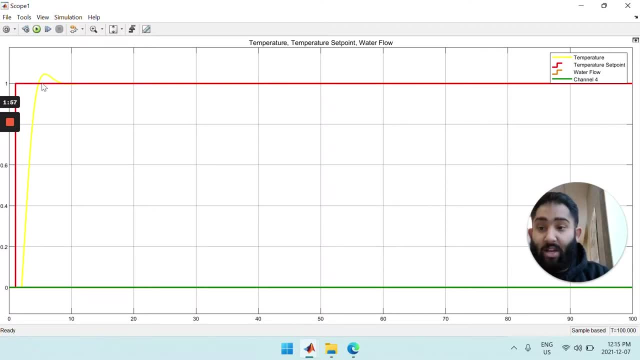 up, jumps up and there is a small overshoot seen over here and the temperature settles within 6 to 7 time units, And this is nice because this allows us to steadily track our temperature of the water. Okay, Regardless of what's occurring, and this allows us to maintain the set point very strictly- 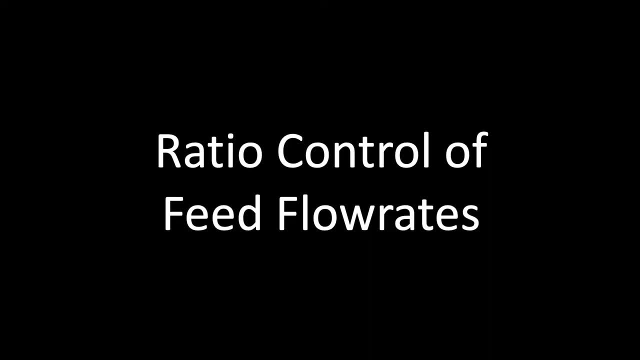 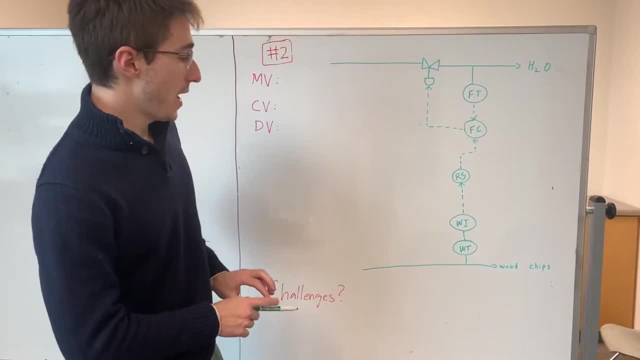 in a short period of time without oscillations. So, taking a look at our P&ID for the ratio control strategy in place, we have two flow streams. We have a water flow as well as wood chip inlet and these serve as the inlet into our 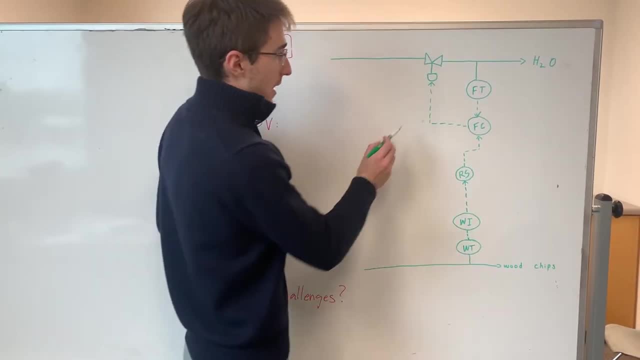 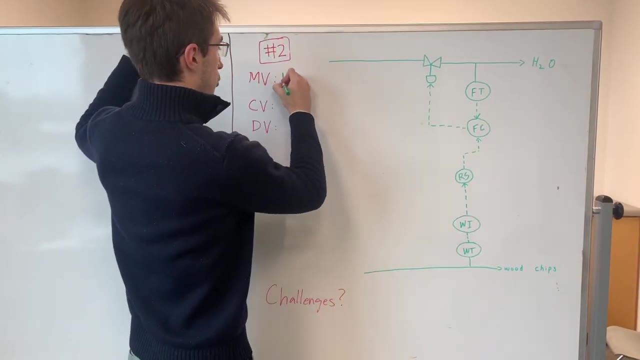 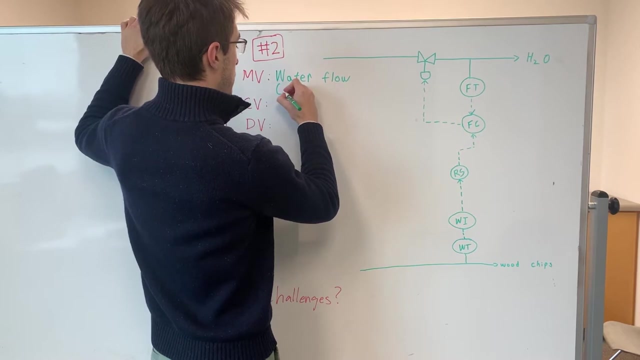 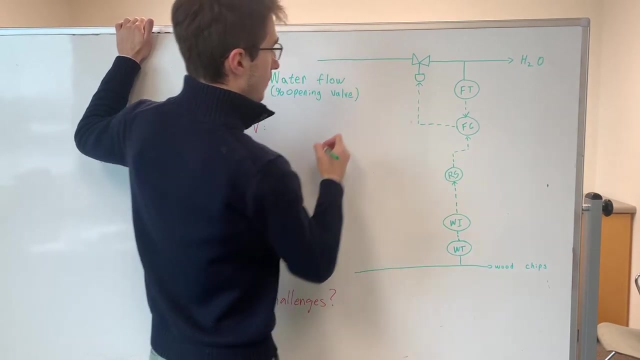 hydrolysis reactor. So here we have a control valve which can be adjusted to manipulate the flow of the water, which is our manipulated variable. So manipulated variable is water flow and we, specifically, are able to manipulate this by adjusting percent opening of the valve. 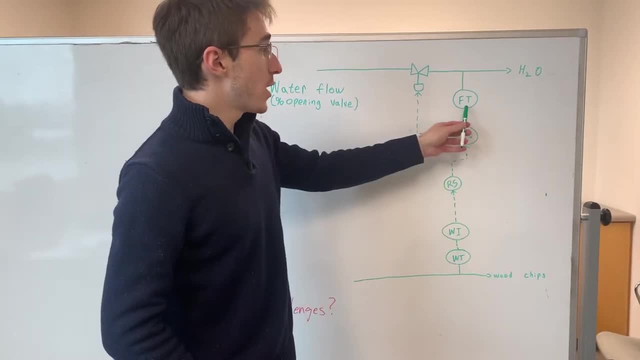 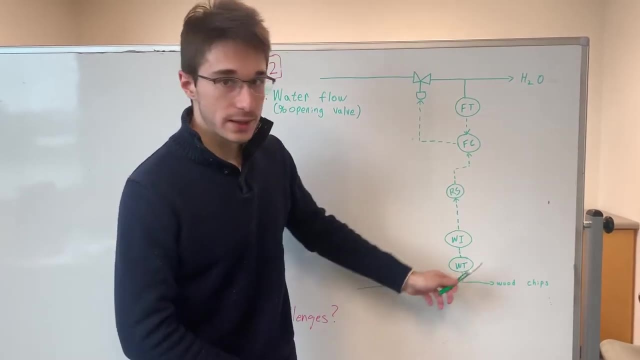 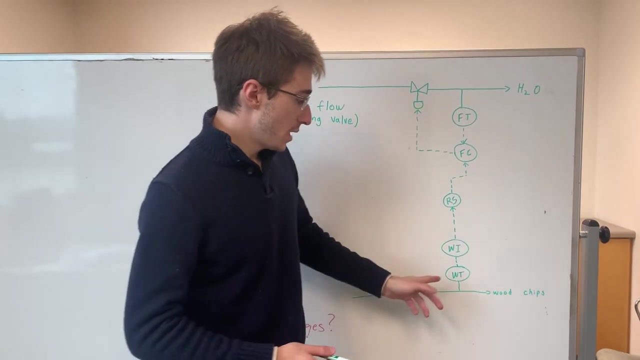 So, again looking at the P&ID, we have a flow transmitter downstream of the valve that feeds into a flow controller On the other side. We're also measuring the weight of the incoming wood chips, and the reason for this is because we're dealing with a solid, so having a flow transmitter wouldn't be as feasible. 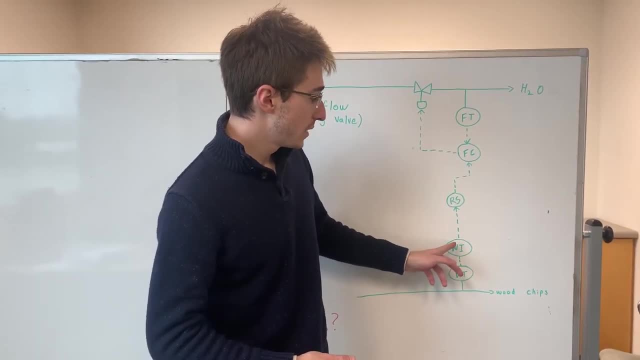 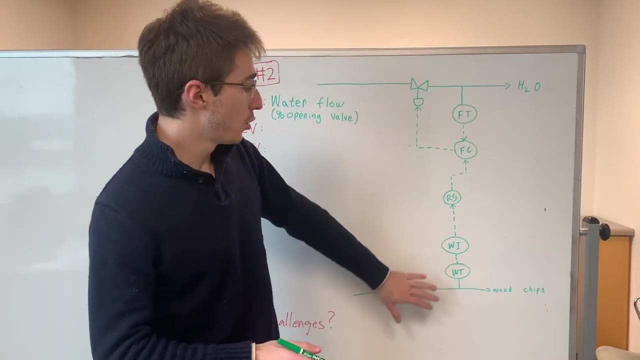 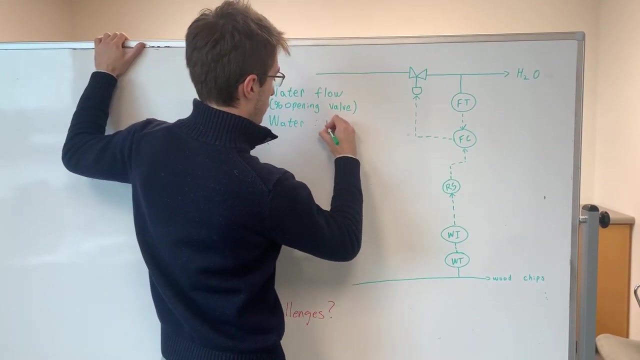 We measure the weight, that is fed into a weight indicator and that goes into the ratio station. So the goal here with this ratio station is to achieve this control of the water to wood ratio. So we have a control variable of a water to wood ratio. 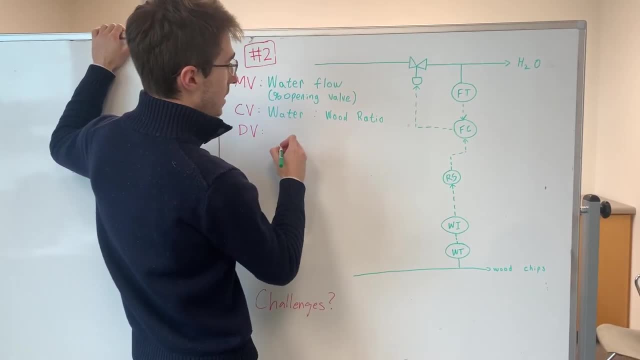 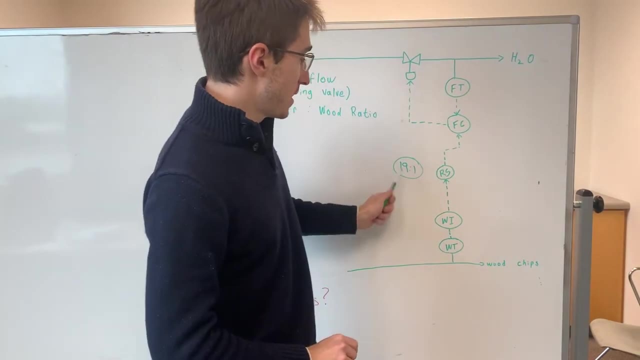 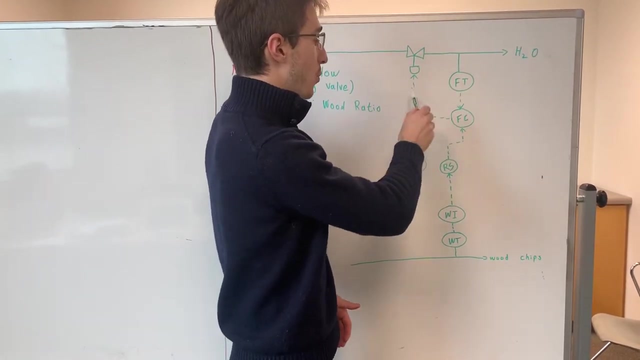 And, as a side note, Literature indicates that this ratio is to be 19 to 1, and this ensures a complete reaction. So the ratio station has a 19 to 1 set point that feeds into the flow controller and, resultantly, we're manipulating this valve opening in order to maintain this ratio. 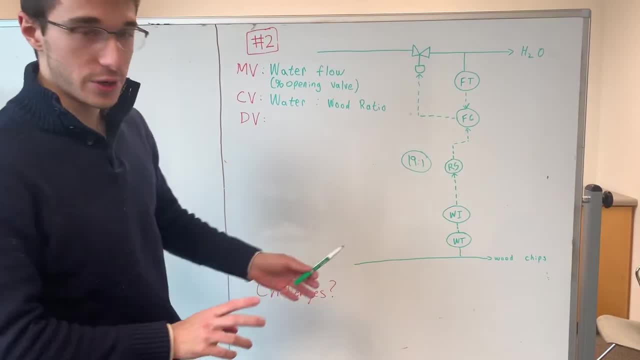 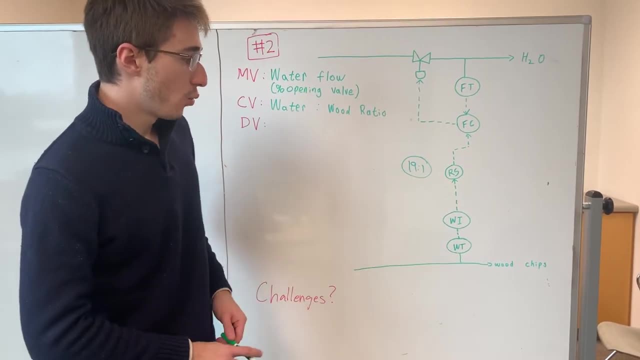 And finally, in terms of disturbances as well as challenges, the primary challenge with this type of process is the variability of the feedstock and wood chips, most notably with wood chips. Wood chips, We're going to be getting different moisture content, as well as potentially different. 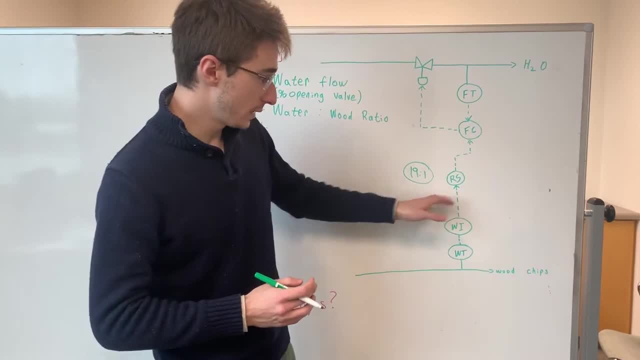 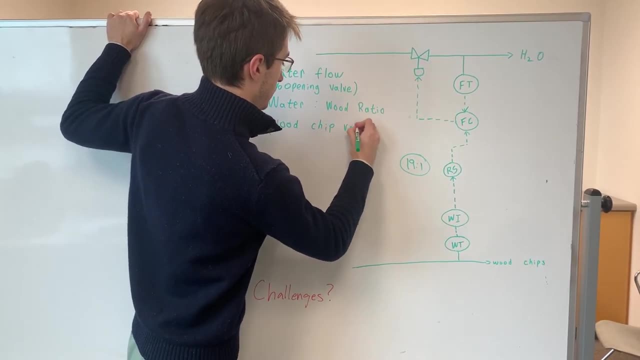 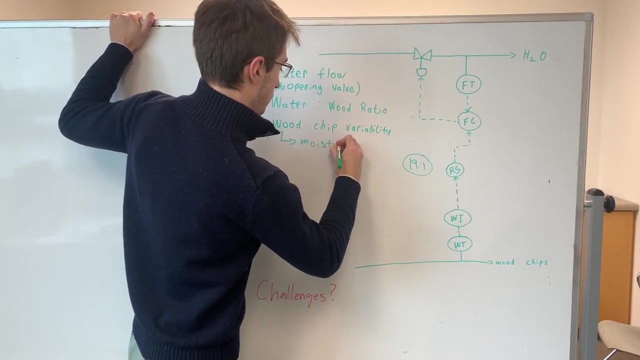 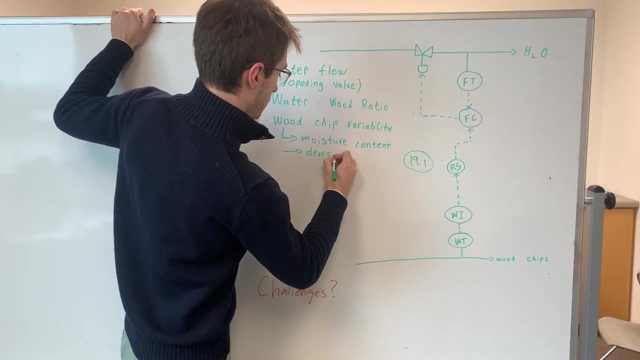 densities. so that makes it difficult to calculate some of the parameters. So deviation variables would be wood chip variability, specifically moisture content as well as density, And this all comes back to the fact that we're dealing with an organic feedstock. so 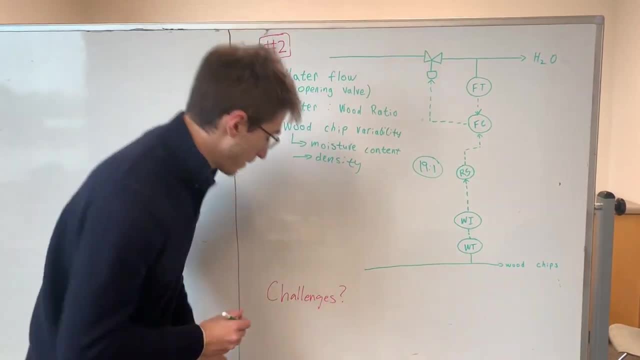 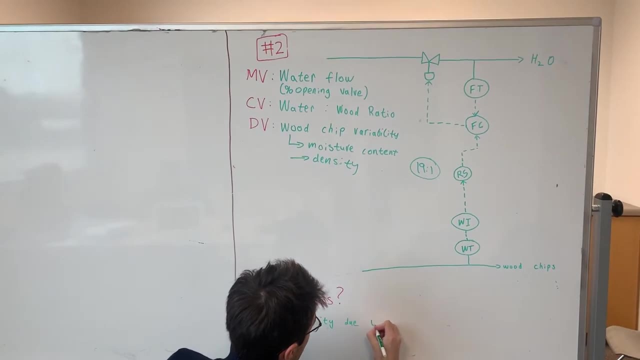 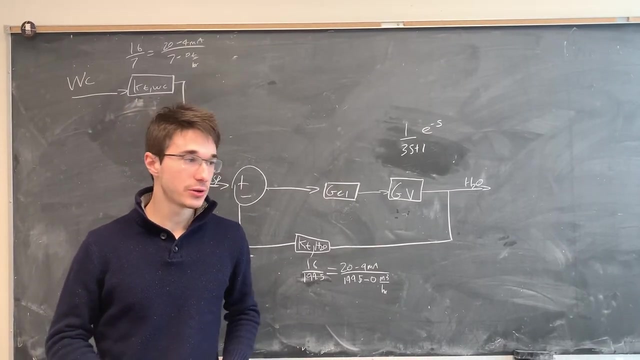 variability is really an inherent factor here. So under challenges we make a note of variability due to natural feedstock. So for our control block diagram, for the ratio control strategy, we have the inlet wood chips And we have the transmitter. Similarly. 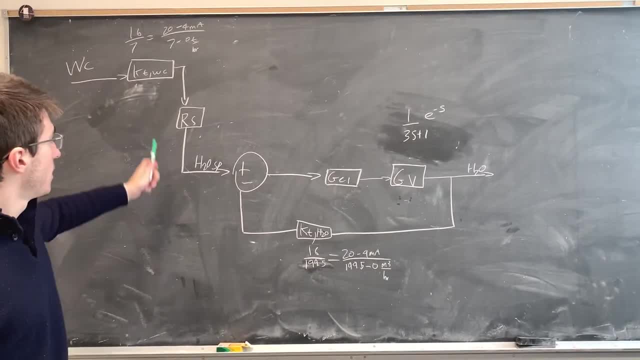 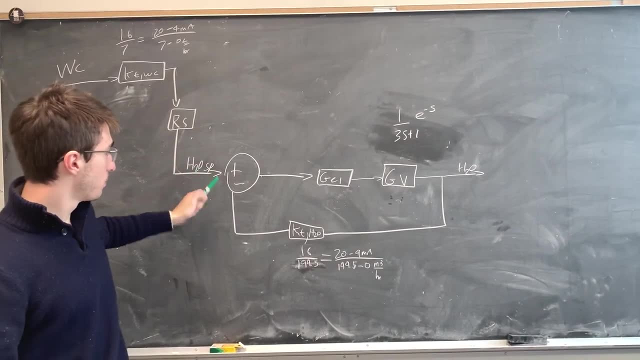 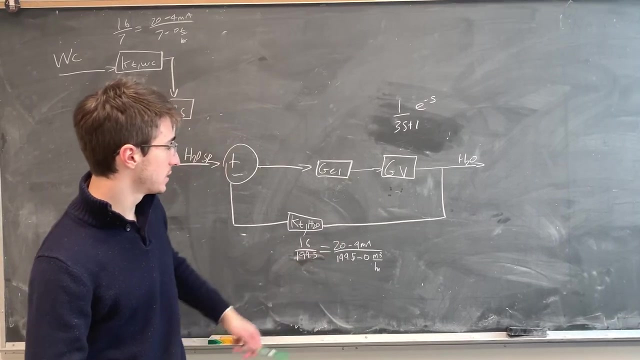 Determined. This is the first control block diagram That feeds into the ratio station, and this is giving us the set point for water flow. We also have a transmitter for water. again similarly determined, we have the electrical output signal as well as the span of the device. 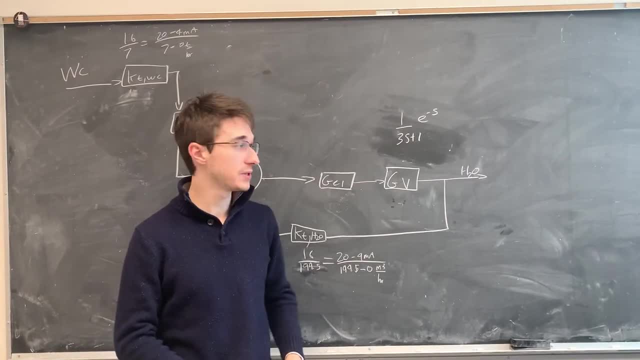 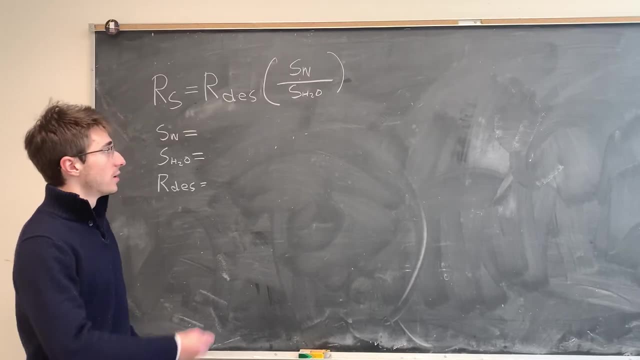 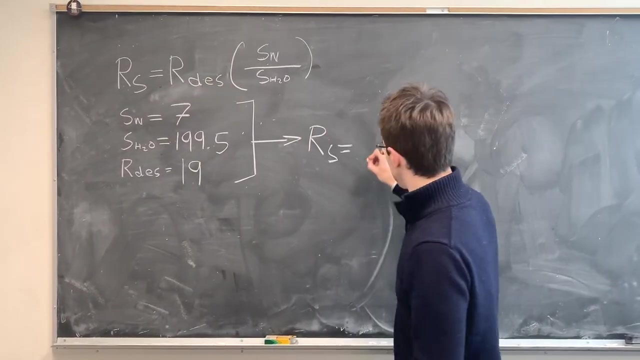 The valve is determined from literature, specifically from the GV474 class notes, and this leaves us with the unknown of the controller, which we will determine shortly. So now let's have a look at the air frequency variable model and see what is going on for 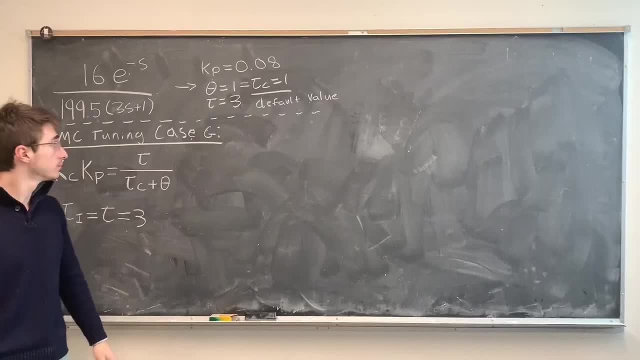 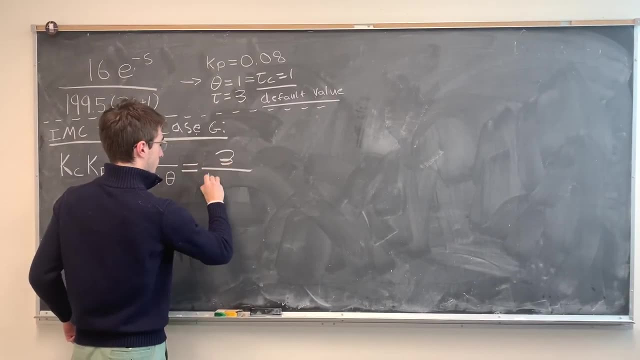 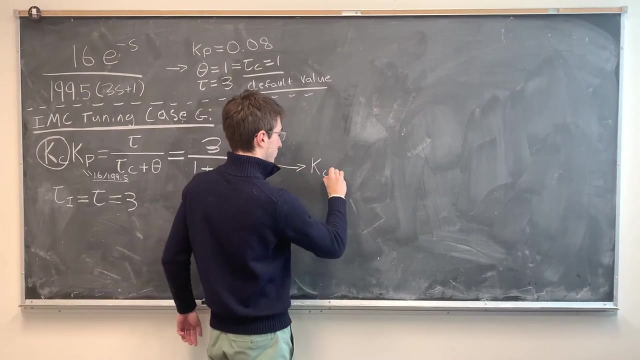 example. So I'll give you the data that's being received and examined. Here's the different values. You can see here that the great difference is the temperature And the difference is the number of weeks, And when you look at the data, it's much lower. 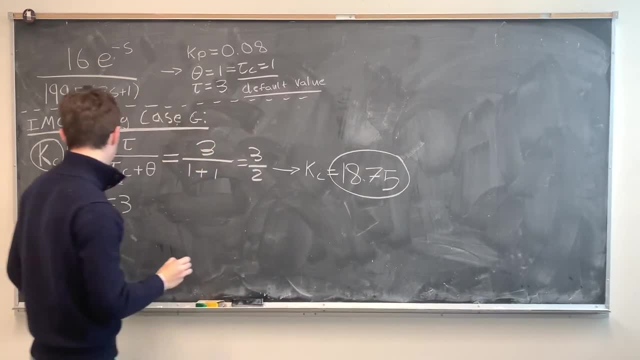 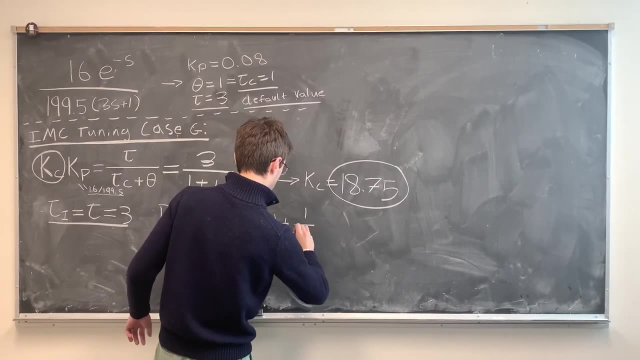 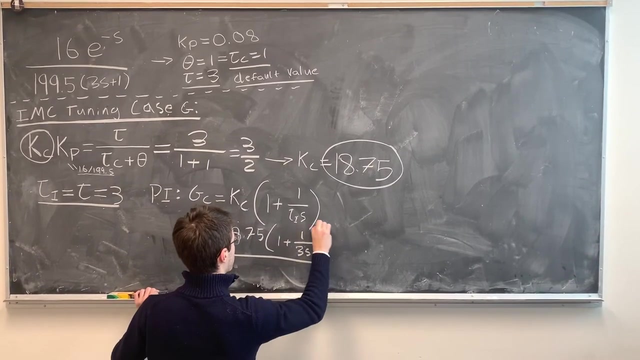 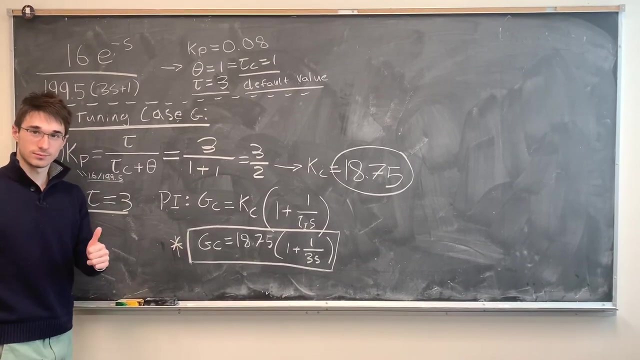 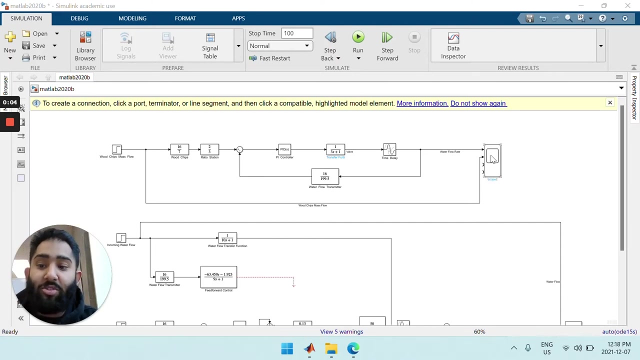 It's about 8 times lower than the current average, So that's why I think it's as good as it is. now on to the other simulink file, which is for ratio control. so we're going to check our step point tracking for the wood chips and see if 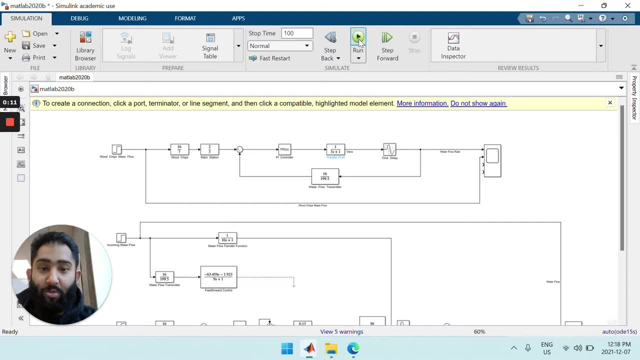 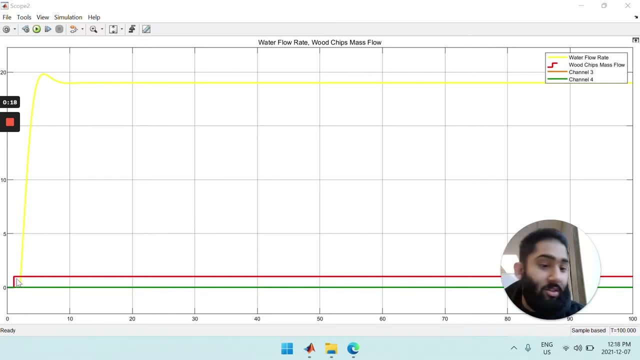 our ratio of wood water to wood chips is tracked properly and over here we can see that there is a step one, a unit step change in the wood chips mass flow and there's a small time delay until the water flow rate follows suit. however, we can see that there is a quick increase in the water flow rate with the small overshoot. the water flow rate is around 20 and then it quickly settles down to the ratio of 19 within seven to eight time units. and this is perfect because operators will change the set point in our process and this allows our water flow rate to follow the ratio that's specified by literature to ensure. 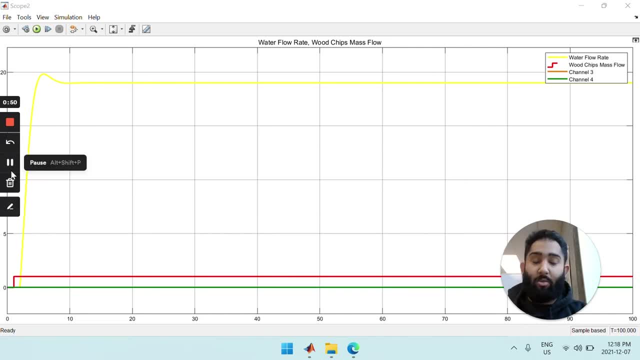 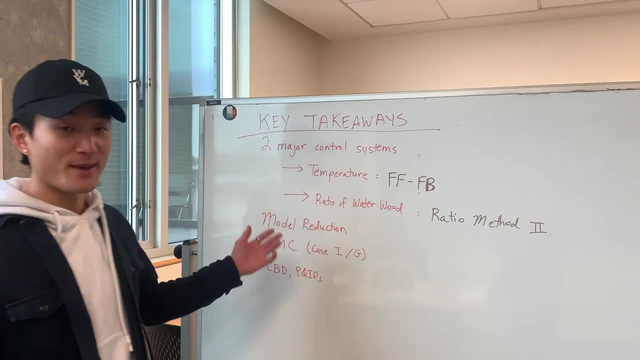 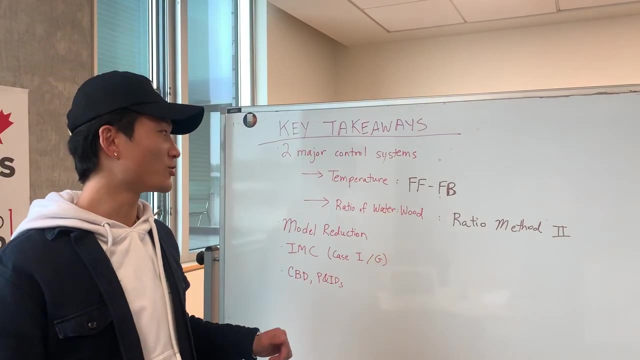 our reaction occurs to completion and our product quality is as expected. so, in conclusion, your main takeaways for this term project. we've selected two major control systems for a capstone project, which include temperature control at 180 degrees Celsius and the ratio of water to wood. 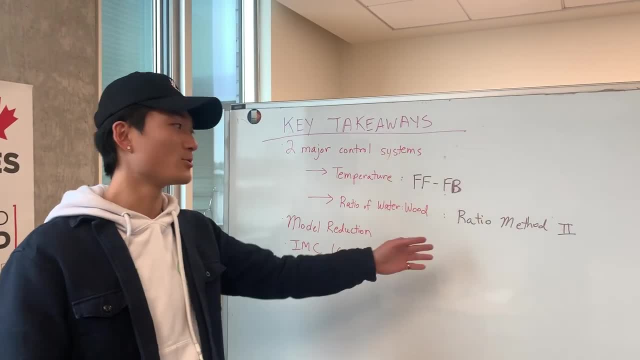 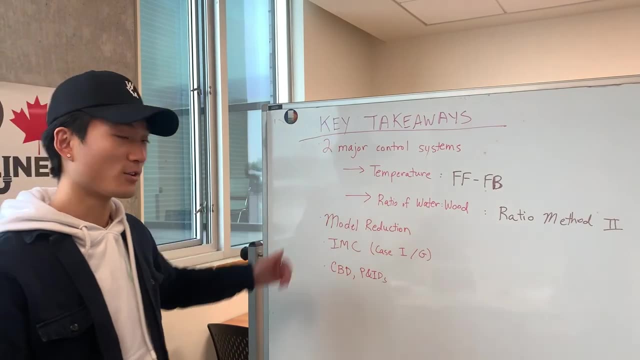 at 19 to 1. we've selected feed forward and feedback, as well as a ratio method 2 for our strategies. the major topics that have been covered in our class that we've covered today include model reduction, IMC cases I and G, as well as. 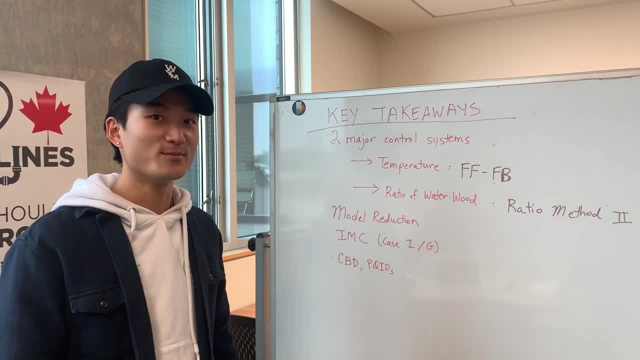 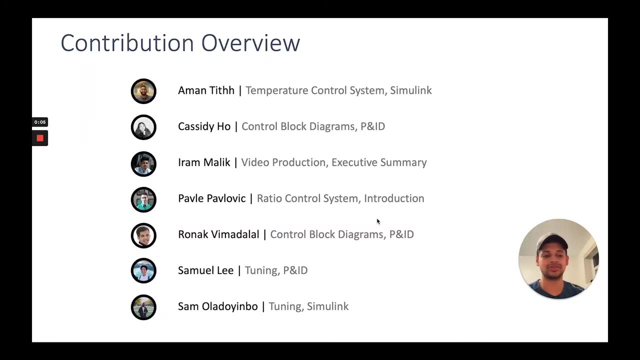 control block diagrams and process and instrumentation diagrams, and with that we want to conclude our presentation. professor, thank you so much for listening in. here's an overview of the contributions of everybody in the team and, as always, stay curious, keep learning and don't forget to smile.